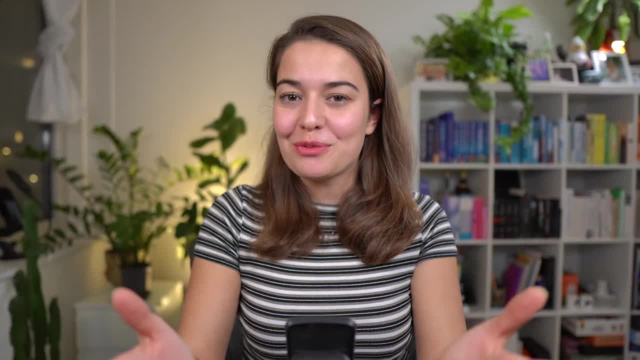 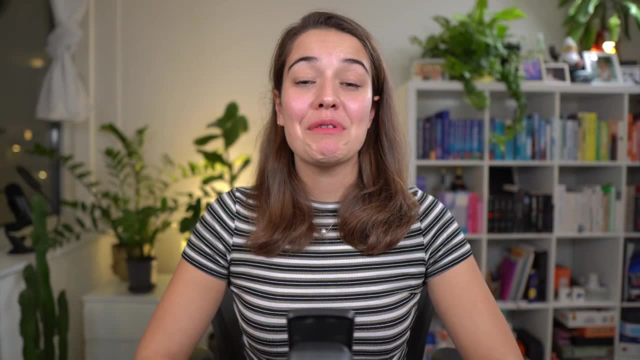 What do you do if your model overfits? Well, regularization, of course, but regularization can be a little bit of a complicated topic. So in this video, we will talk about regularization. We will talk about what regularization is, how and why it works for neural networks. 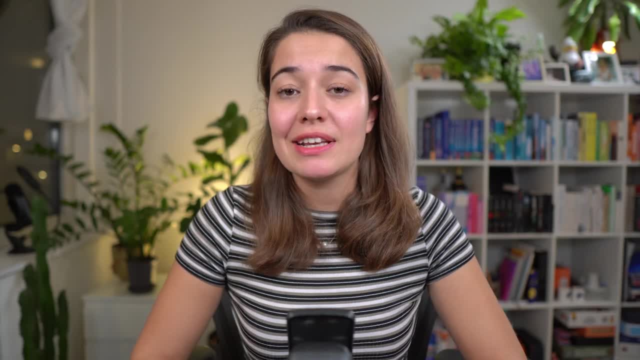 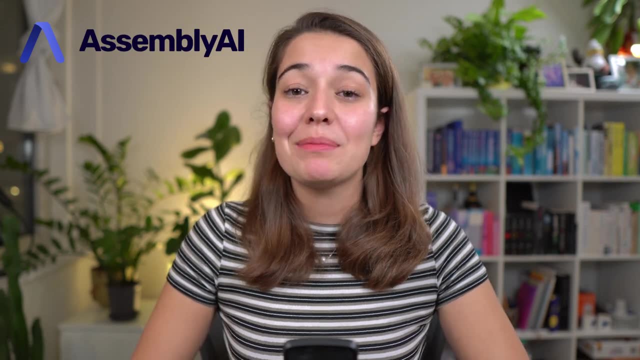 and we will go into details of some of the regularization techniques, like L1, L2, and dropout regularization. This video is part of the Deep Learning Explained series by Assembly AI. Assembly AI is a company that is making a state-of-the-art speech-to-text API. 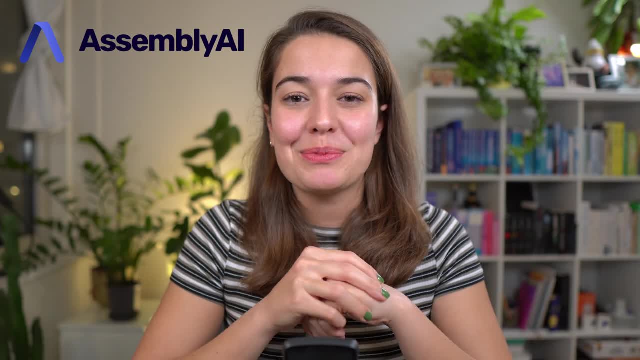 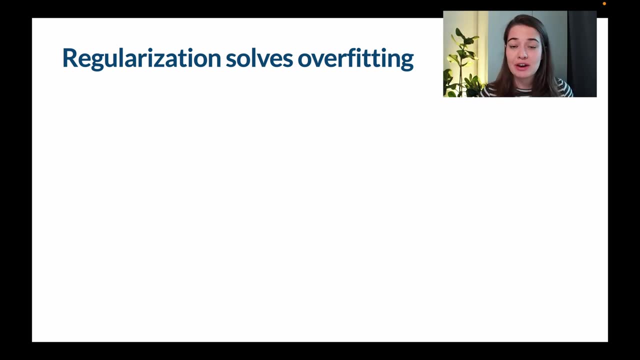 If you also want to get a free API token, use the link in the description. Why do we use regularization? We use regularization for overfitting. We use regularization to fix overfitting in our neural networks or other machine learning models. So what is overfitting? 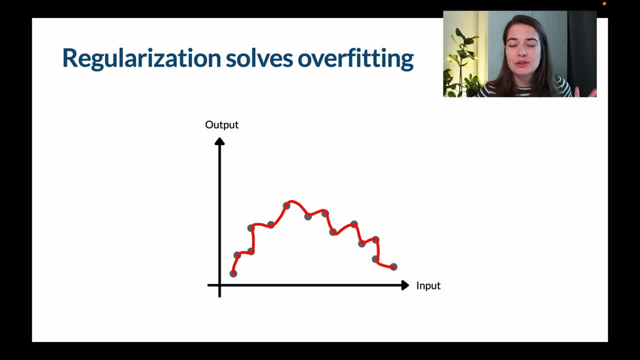 Overfitting is when your model really closely fits the training data, so much so that it is not able to generalize really well to the real world. So if you look at the example, if we have only one input and we have only one output, an overfitted model would look. 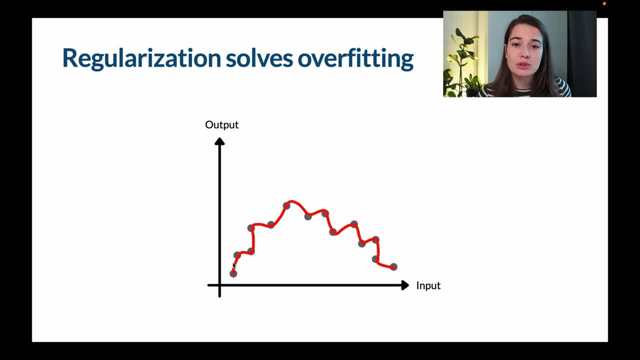 something like this: It really closely follows all the input values and believes that this perfectly summarizes the real world, whereas that's not really the case, of course. How can you understand if your model has overfitting or not? Well, we do that by looking. 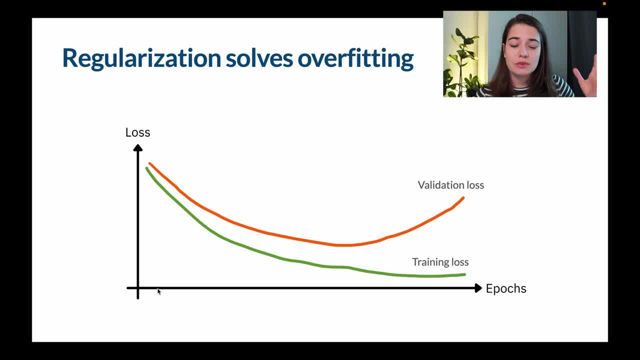 at the difference between validation loss and training loss. We will look at as we train. our model more and more is we use more epochs. After some time, validation loss will start getting higher, whereas the training loss keeps getting lower and lower, And we know from that point on we started to overfit. 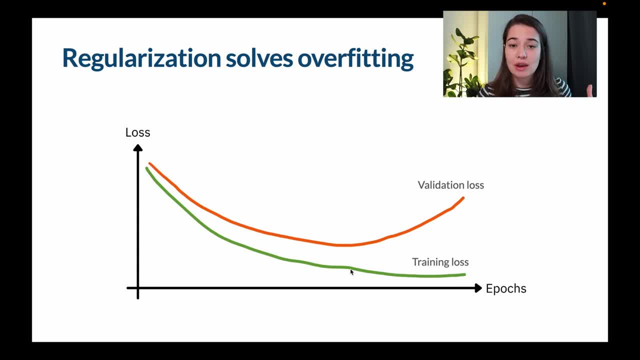 because our model learns more closely what is being represented in the training data set, whereas it is not able to really understand what's going on with the validation data set or generally in the real world. It is not really able to understand the pattern and the data. 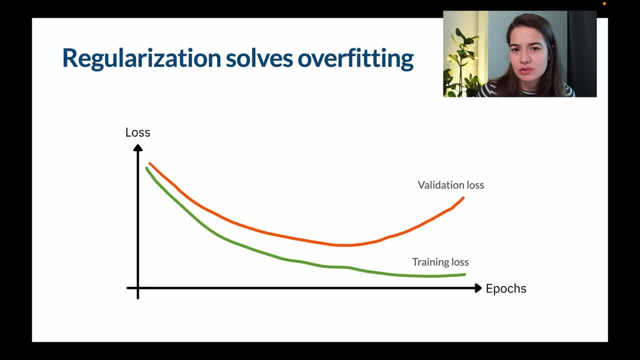 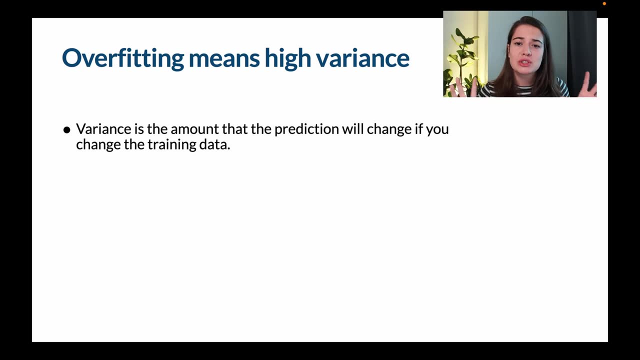 well anymore. But how can regularization solve this? So let's take one step back and understand what happens when your model is overfitting. When your model is overfitting, it means that your model has high variance. Let's remember what variance is. It is basically how much your predictions will. 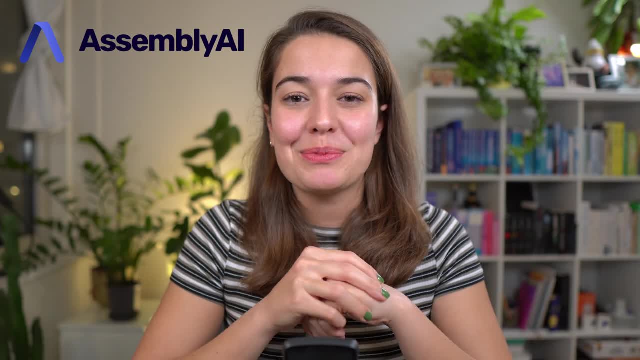 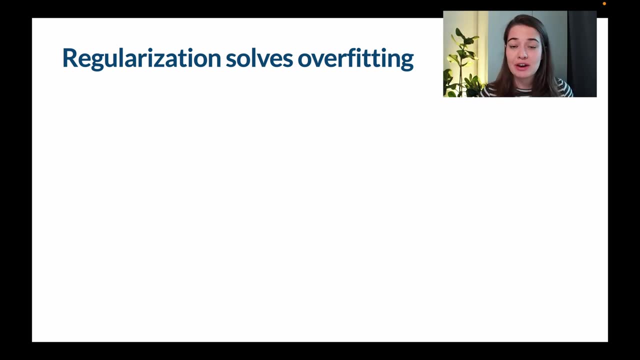 If you also want to get a free API token, use the link in the description. Why do we use regularization? We use regularization for overfitting. We use regularization to fix overfitting in our neural networks or other machine learning models. So what is overfitting? 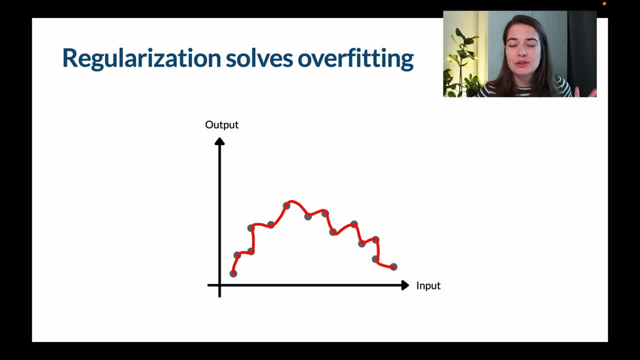 Overfitting is when your model really closely fits the training data, so much so that it is not able to generalize really well to the real world. So if you look at the example, if we have only one input and we have only one output, an overfitted model would look. 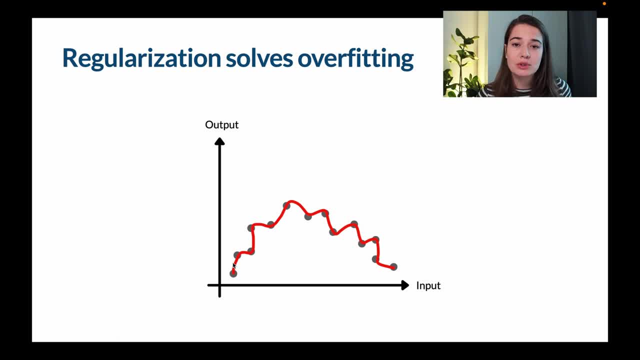 something like this: It really closely follows all the input values and believes that this perfectly summarizes the real world, whereas that's not really the case, of course. How can you understand if your model has overfitting or not? Well, we do that by looking. 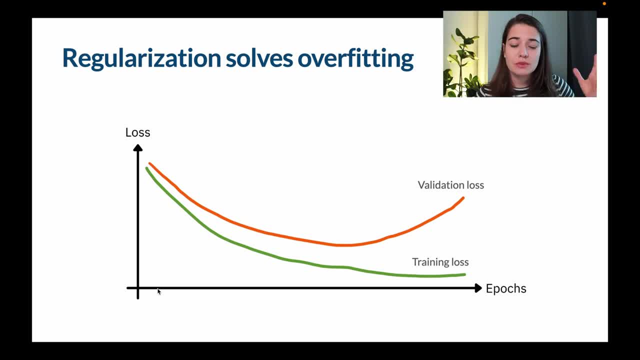 at the difference between validation loss and training loss. We will look at as we train our model more and more. If we train our model more and more, we will look at the difference between validation loss and training loss more. if, as we use more epochs, after some time validation loss will start getting higher, whereas 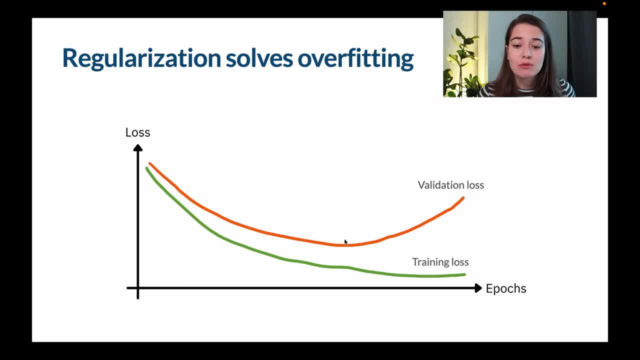 the training loss is getting, keeps getting lower and lower and we know from that point on we started to overfit, because our model learns more closely what is being represented in the training data set, whereas it is not able to really understand what's going on with the validation data set. 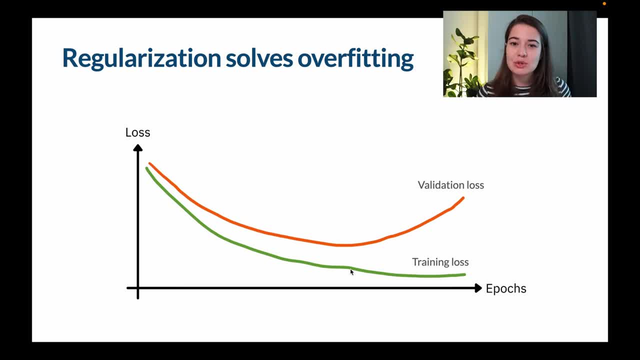 or generally, in the real world, it is not really able to understand the pattern and the data well anymore. but how can regularization solve this? so let's take one step back and understand what happens when your model is overfitting. when your model is overfitting, it means that your model 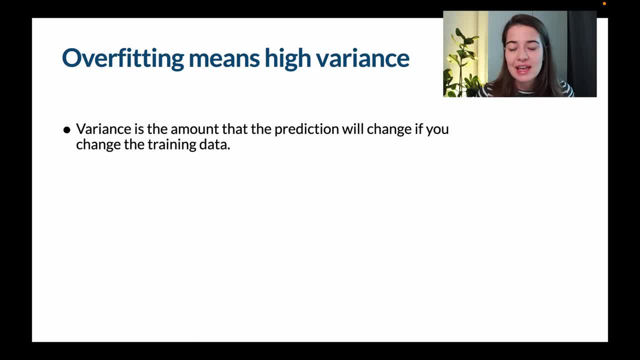 has high variance. let's remember what variance is. it is basically how much your predictions will change on your model if the training data that you're training your model with changes a little bit. so that is, how sensitive is your model on the training data that you're giving it to? because if 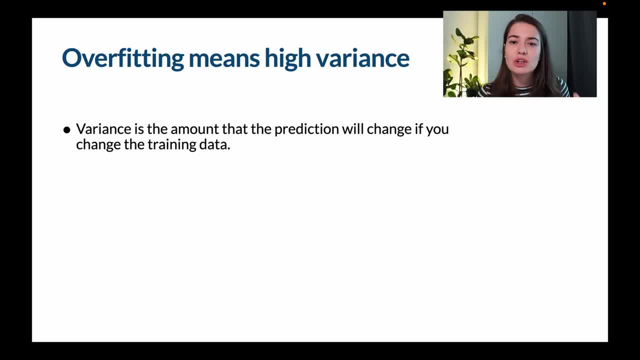 it's more sensitive. it's more sensitive to the training data that you're giving it to. it means that it is overfitting. but what causes this high variance? well, one thing that causes high variance is the flexibility of the models, because the more parameters that you have in 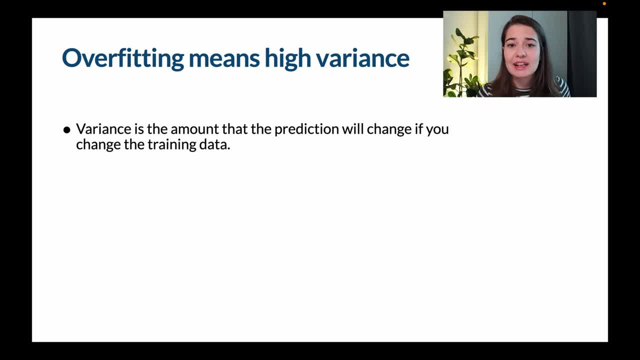 change on your model if the training data that you're training your model with changes a little bit. So that is, how sensitive is your model on the training data that you're giving it to? Because if it's more sensitive, it's more sensitive to the training data that you're giving it to. So that's. 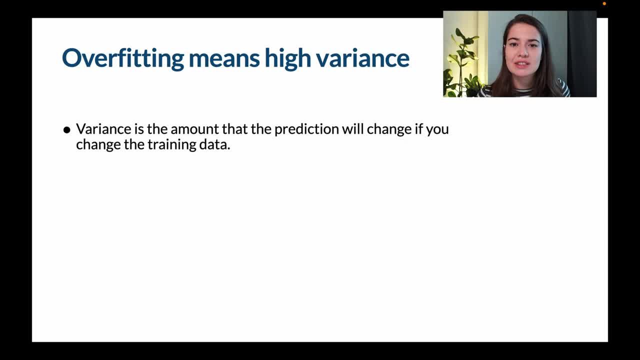 it means that it is overfitting. But what causes this high variance? Well, one thing that causes high variance is the flexibility of the models, Because the more parameters that you have in your model, the more flexibility, the more things that you can tweak in your model, it is more likely that 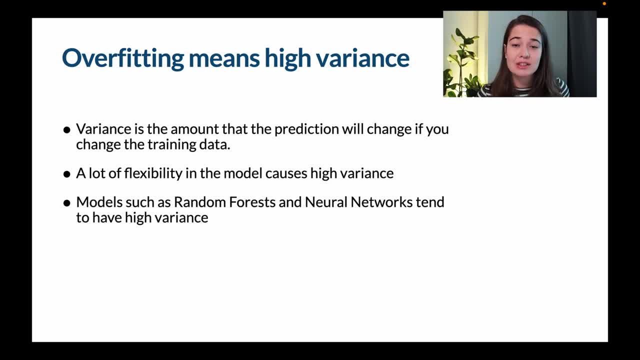 you will have high variance. Some examples of models that have high variance or high flexibility and thus high variance, are random forests or neural networks, for example, And that's exactly where regularization comes in. Regularization is a way to limit this flexibility that the model has. 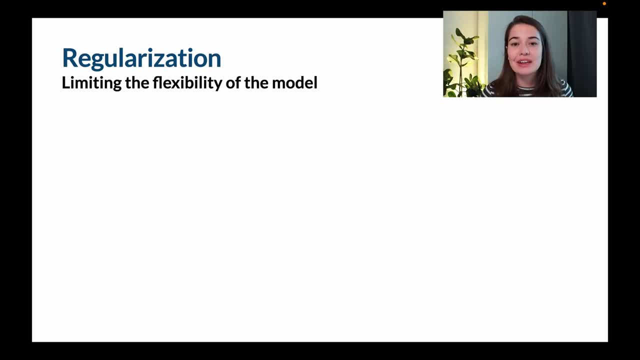 in hopes to avoid overfitting. This could be done in a bunch of different ways, But for neural networks specifically, this means to lower the weights of the network. You might be asking, of course, what does high weights have anything to do with overfitting? Well, let's look into that now. 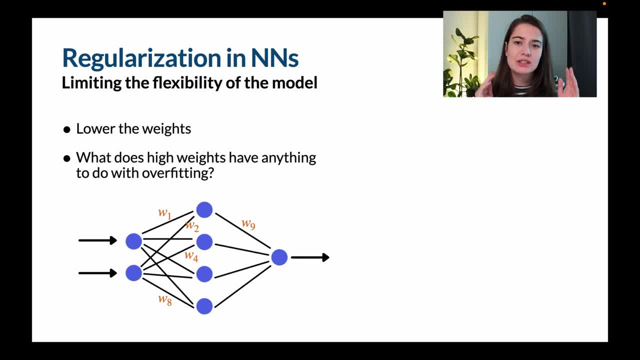 So let's take this example. Let's say we have this neural network, it has one hidden layer and it has four neurons, And in all of these connecting connections between the neurons we have weights. What does those weights mean? What are those weights? Well, let's take a look. 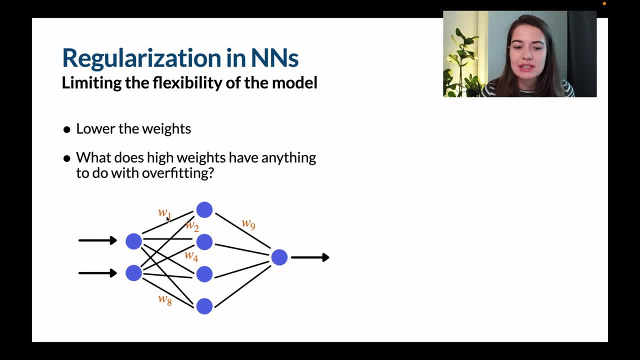 What are they signifying? So, when you think about it, these weights are basically the importance of the output of the certain neuron. So if it's right after the input layer, it means the importance of this input. If it's in between, in the hidden layers, it means the importance of the output. 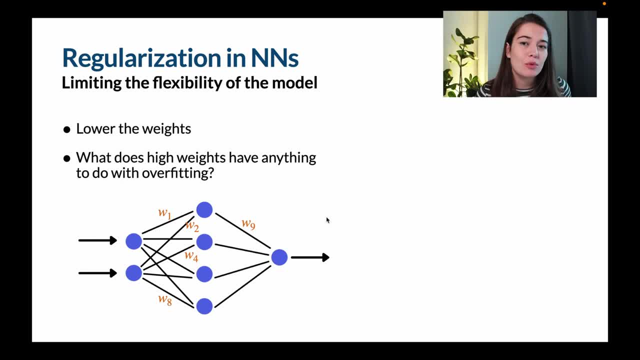 of this neuron And let's look back at an example of what it looks like when we are overfitting. If we have only one input and only one output, what happens is the model that we're training the function really closely follows. 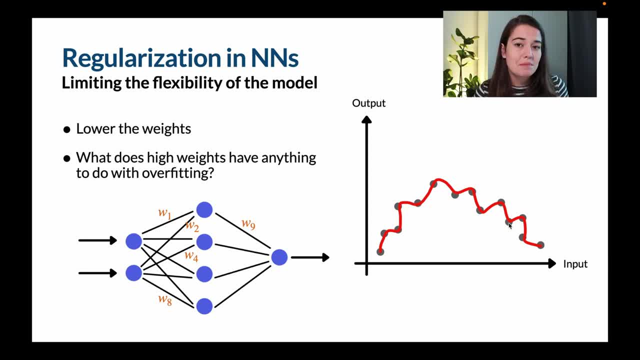 what the input values are. So what that means is that when you're overfitting, you're exaggerating the importance of a certain input or for a certain data point. And how can you do that in a neural network If you have a really high weights for a certain input or a certain data point? that would 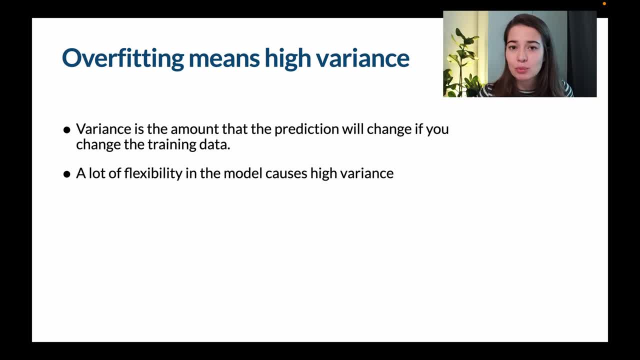 your model. the more flexibility, the more things that you can tweak in your model, it is more likely that you will have high variance. some examples of models that have high variance or high flexibility and thus high variance are random forest or neural networks, for example, and that's exactly where 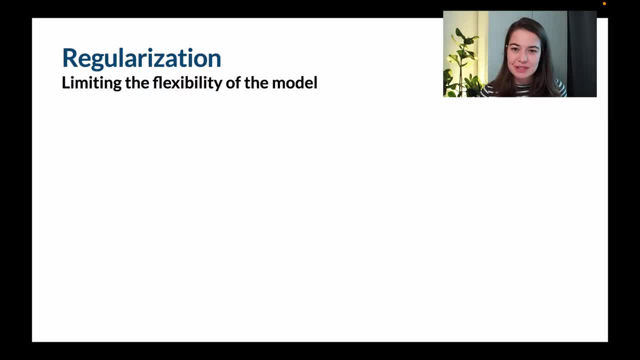 regularization comes in. regularization is a way to limit this flexibility that the model has in hopes to avoid overfitting. this could be done in a bunch of different ways, but for neural networks specifically, this means to lower the weights of the network. you might be asking, of course, what? 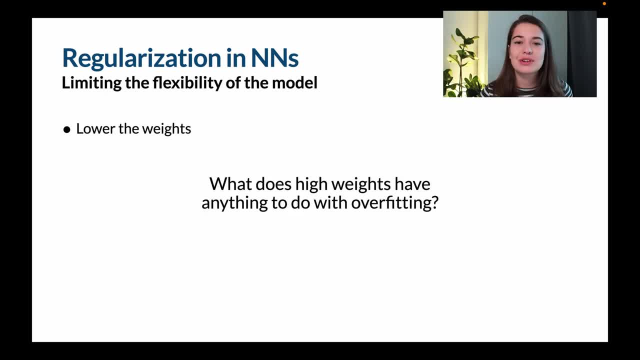 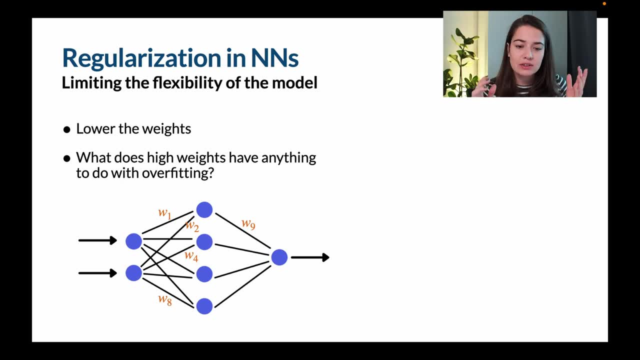 does high weights have anything to do with overfitting? well, let's look into that now. so let's take this example. let's say we have this neural network. it has one hidden layer and it has four neurons, and in all of these connecting connections between the neurons we have weights. what does those 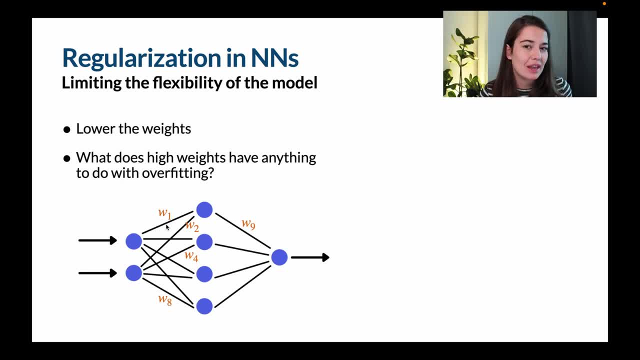 weights mean. what does that mean and what does that mean, and what does that mean and what does that mean? what is, what are they signifying? so, when you think about it, these weights are basically the importance of this, the output of the certain neuron. so, if it's right after the input layer. 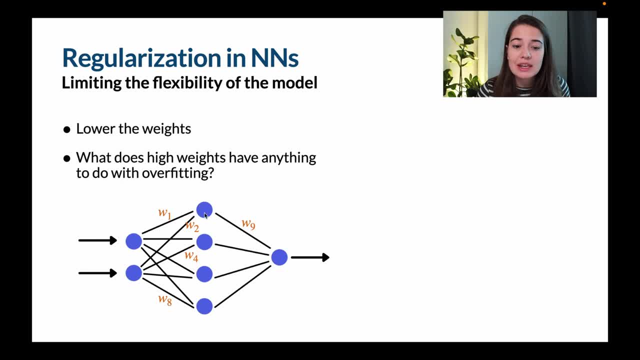 it means the importance of this input if it's in between, in the hidden layers. it means the importance of the output of this neuron. and let's look back at an example of what it looks like when we are overfitting. if we have only one input and only one output, what happens is the nerve, the 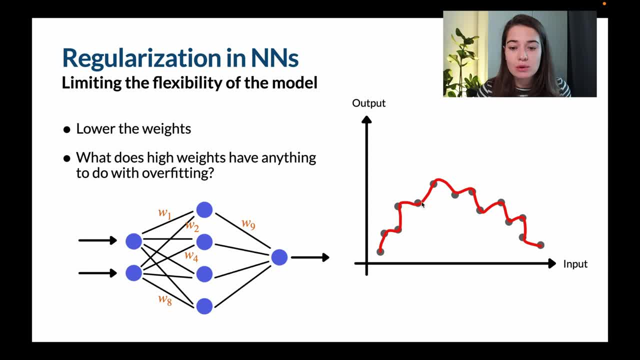 model that we're training, the function really closely follows the output of the certain neuron. so what that means is that when you're overfitting, you're exaggerating the importance of a certain input, of a certain data point. and how can you do that in a neural network if you have a really high? 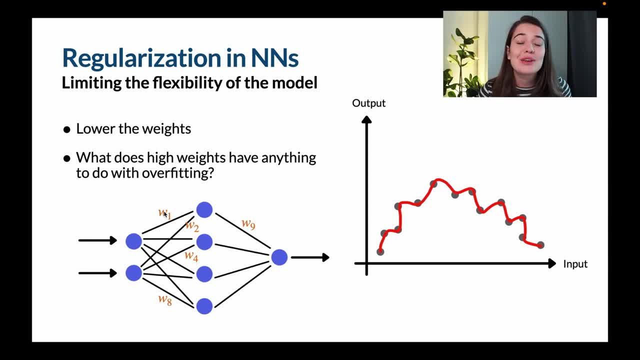 weight for a certain input or a certain data point. that would mean that you're exaggerating the importance of that data point. so how can you avoid this if you lowered the weights? so that's why, while we are fighting with overfitting in neural networks, what we aim to do with 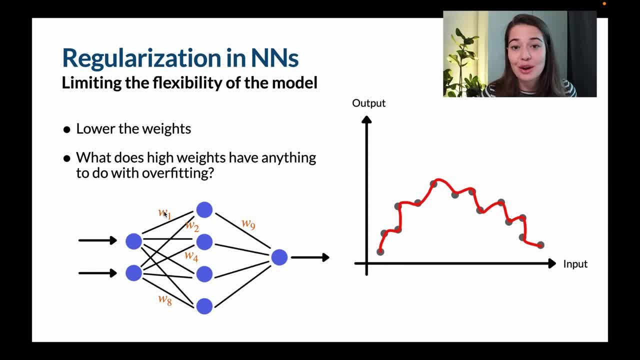 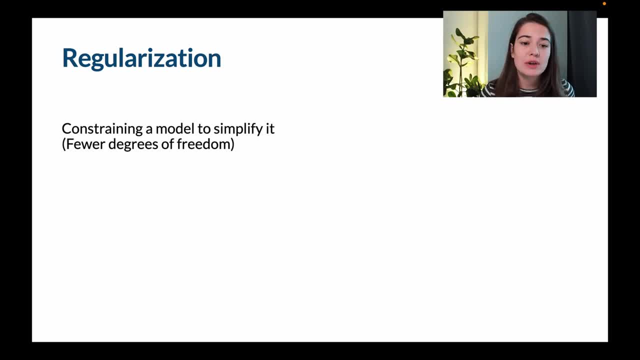 regularization is to lower the weights that we have in the neural network. let's see what type of solutions we have in the regularization. so there are two types of regularization techniques. the first one is, as we talked about, constraining the model, the constraining, the flexibility of the 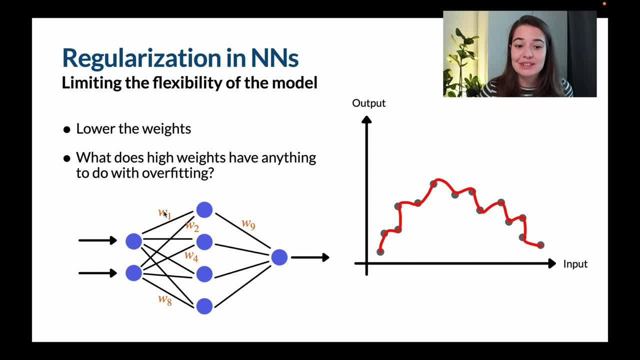 mean that you're exaggerating the importance of that data point. So how can you avoid this if you lower the weights. So that's why, while we're fighting with overfitting in neural networks, what we aim to do with regularization is to lower the weights that we have in the neural network. 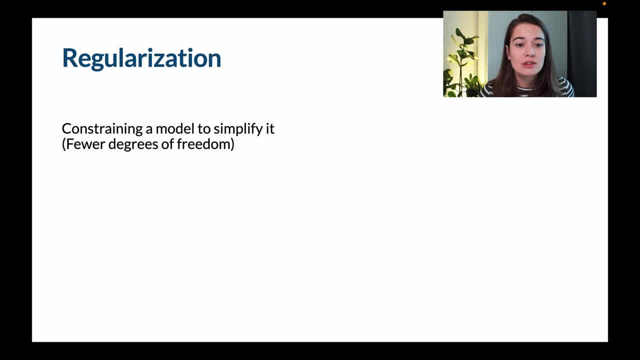 Let's see what type of solutions we have in the regularization. So there are two types of regularization techniques. The first one is, as we talked about, constraining the model, the constraining, the flexibility of the model, or you could call it. then we have fewer degrees of freedom And the options to do that is either using L1 or L2. 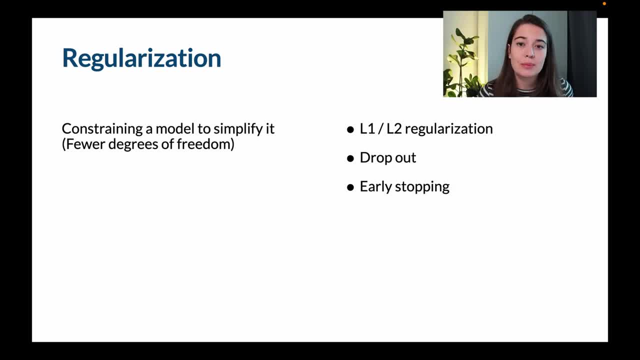 regularization. dropout regularization or early stopping. That's another option that you can use. Another thing you can do is to lower the weights that we have in the neural network. You can use to avoid overfitting and kind of it's in the also the bag of regularization. 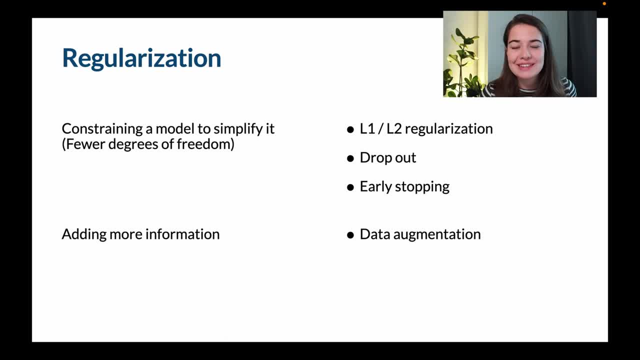 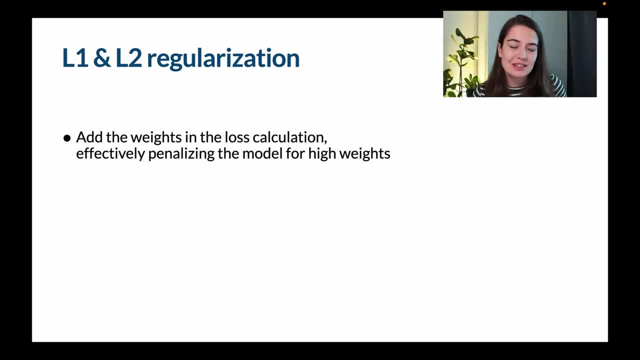 is using data augmentation, So let's go one by one on these techniques and see how they work. The idea behind L1 and L2 regularization is to adding the weights into the loss calculation or the cost function to punish the network for having higher weights. They just have slightly. 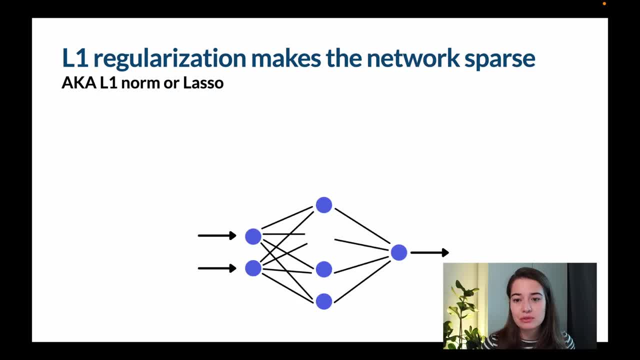 different approaches of how they do this. So when you're using L1 regularization, you can also see it to mention this L1 norm or lasso all over the internet or in the sources that you're looking into. You are adding the sum of the absolute values of the weights to the loss, So it doesn't 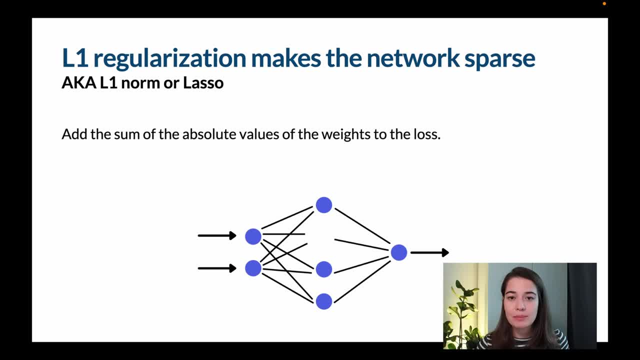 matter if your weights are negative or positive. you sum them all up using the absolute values and then you add it to the cost, And what happens is, as a result, L1 regularization encourages the network to have weights as low as zero. And what happens when you have weights as low as zero? That 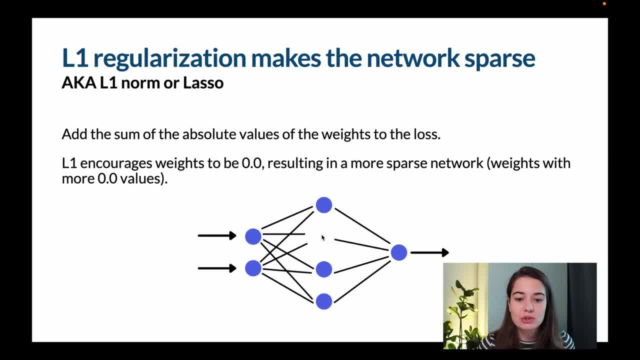 is, some of the outputs will not even be considered in the network calculation. So it might look like this: even though you used to have four neurons in this hidden layer, Because this connection is now zero, this neuron is basically not really looked into yet, So, as a result, you might end up with a 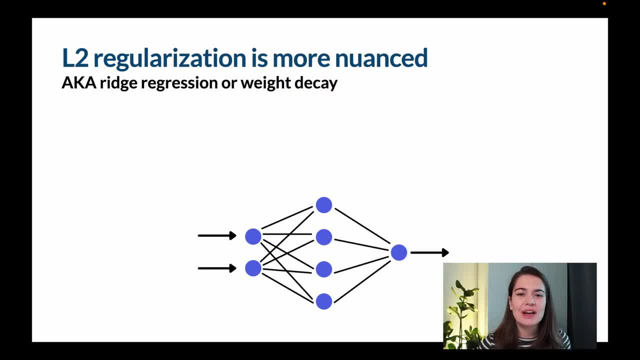 more sparse network. L2 regularization is a little bit more different. Again, you might see it mentioned as ridge regression or weight decay, all over the sources that you might find, And here what we do is we get the sum again of the weights, but they're squared values. So again you're basically making the negative ones. 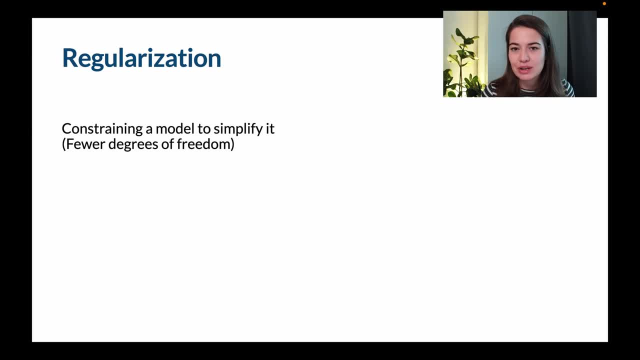 model, or you could call it. then we have fewer degrees of freedom and the options to do that is either using l1 or l2 regularization, dropout regularization or early stopping. that's another option that you can use. another thing you can do is to lower the weights of the neural network. 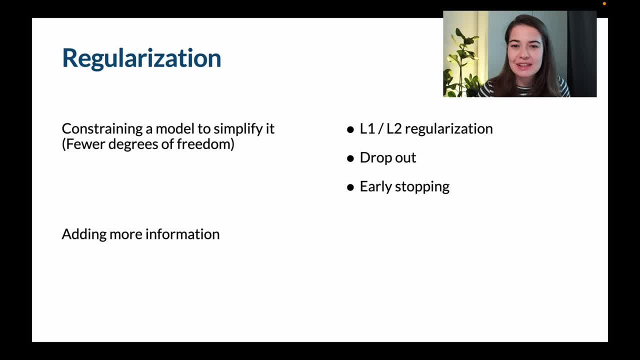 you can use to avoid overfitting and kind of it's in the. also, the bag of regularization is using data augmentation. so let's go one by one on these techniques and see how they work. the idea behind l1 and l2 regularization is to adding the weights into the loss calculation or the cost function. 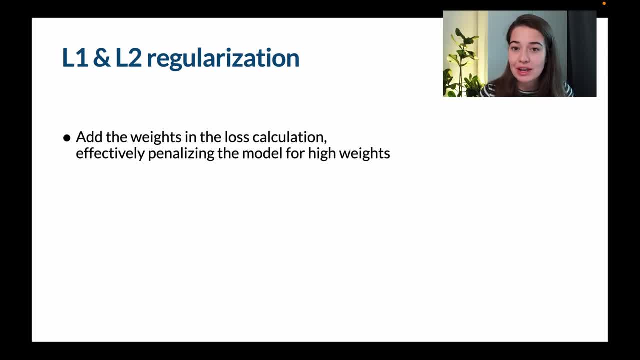 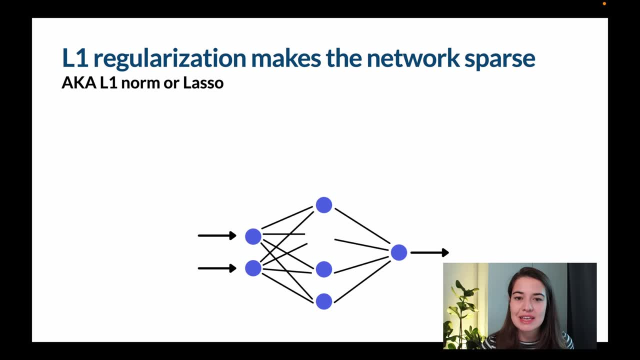 to punish the network for having higher weights. they just have slightly different approaches of how they do this. so when you're using l1 regularization, you can also see it mentioned as l1 norm or lasso all over the internet or in the sources that you're looking. 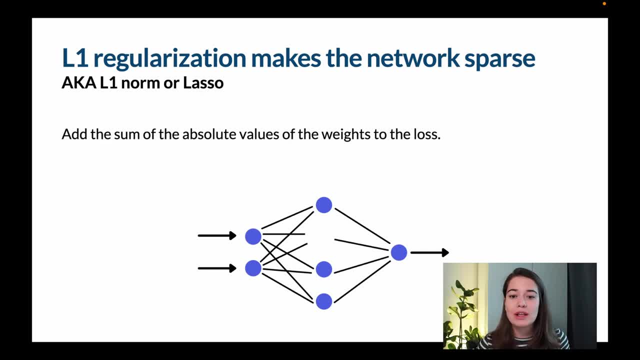 into. you are adding the sum of the absolute values of the weights to the loss. so it doesn't matter if your weights are negative or positive. you sum them all up using the absolute values and then you add it to the cost and what happens is as a result: l1: regularization encourages the 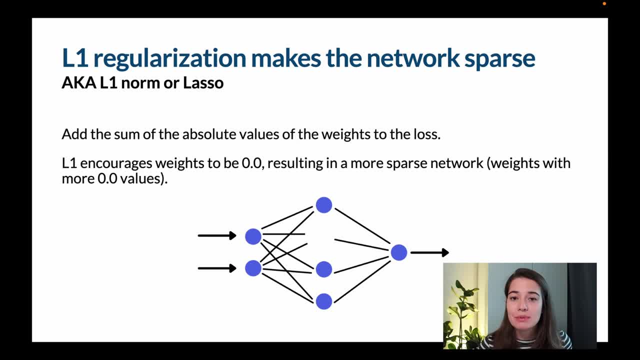 network to have weights as low as zero. and what happens when you have weights as low as zero? that might mean that some of the weights that you're adding to the loss calculation are negative and some of the outputs will not even be considered in the network calculation. so it might 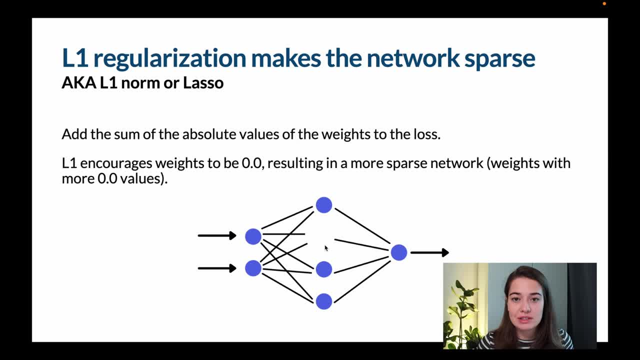 look like this, even though you used to have four neurons in this hidden layer, because this connection is now zero, this neuron is basically not really looked into yet, so as a result, you might end up with a more sparse network. l2 regularization is a little bit more different. 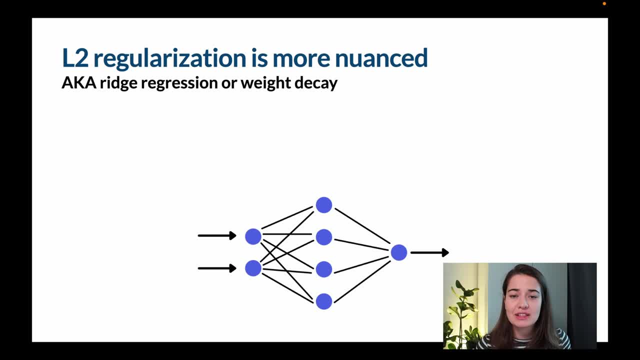 again, you might see it mentioned as ridge regression or weight decay, all over the sources that you might find. and here what we do is we get the sum again of all the weights, but they're squared values. so again you're basically making the negative ones positive, but at the same time you're exaggerating the effects of the higher values compared to the. 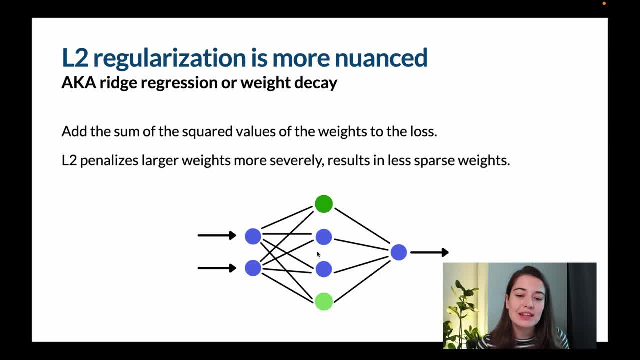 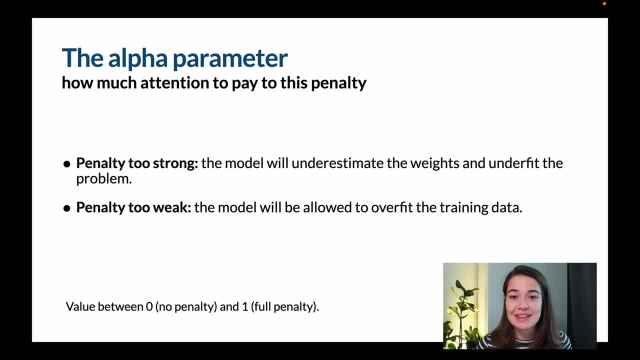 lower values and, as a result, you're going to have differences in the weights of the network, but you're not really going to have a sparse network at the end of l2 regularization. both of these techniques- l1 and l2 regularization- have a parameter called alpha that you need to tune. what alpha does is determines how much attention to 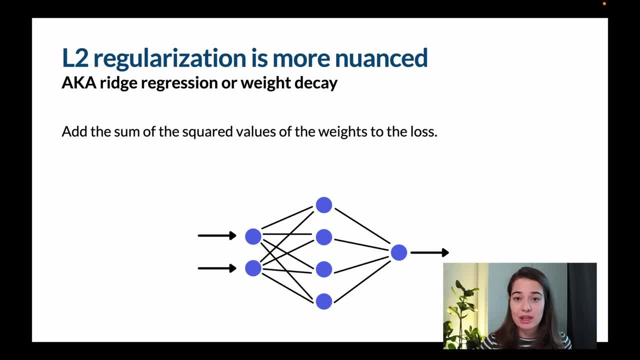 positive, but at the same time, you're exaggerating the effects of the higher values compared to the lower values And, as a result, you're going to have differences in the weights of the network, but you're not really going to have a sparse network at the end of L2. 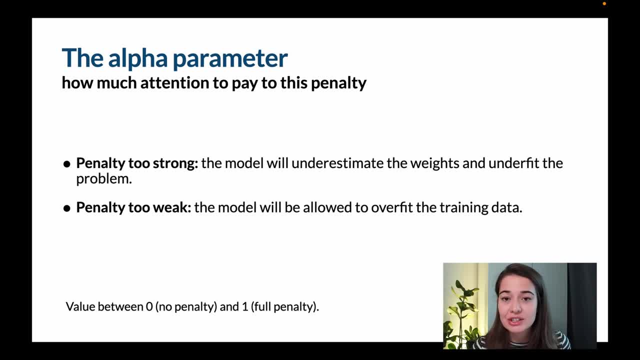 regularization. Both of these techniques- L1 and L2 regularization- have a parameter called alpha that you need to tune. What alpha does is determines how much attention you pay to this penalty. So for L1, it was just the sum of all the weights. 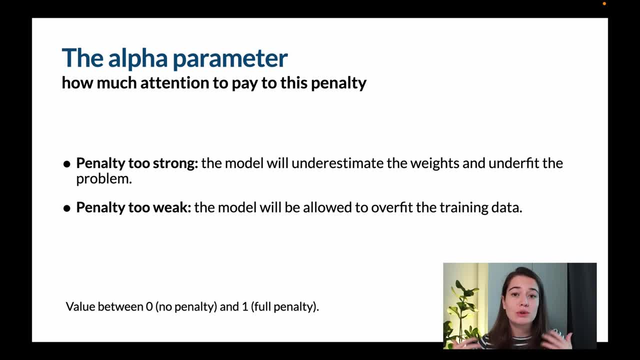 the absolute values of weights. For L2, it was the squared values of the weights. sum of squared values of the weight. So this alpha parameter tells us how much attention to pay to this penalty. If you make the penalty too strong, then you're going to be regularizing. 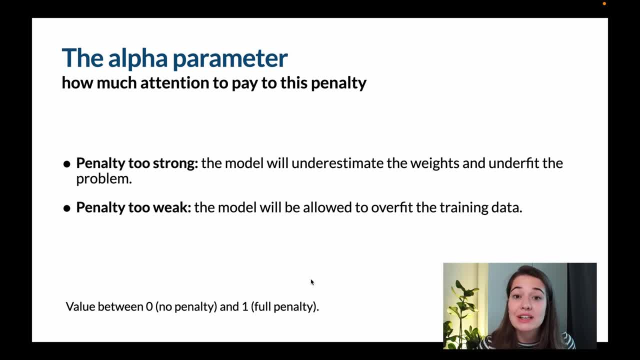 a little bit too hard, and it is likely that your model might underfit your model. While you're trying to avoid overfit, you might get caught in underfitting. If you make the penalty too weak, though, then your model will be allowed to. 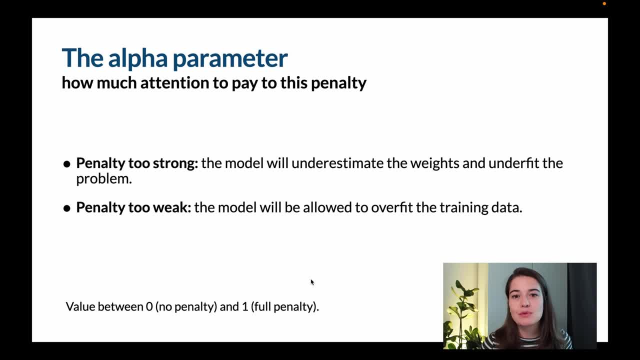 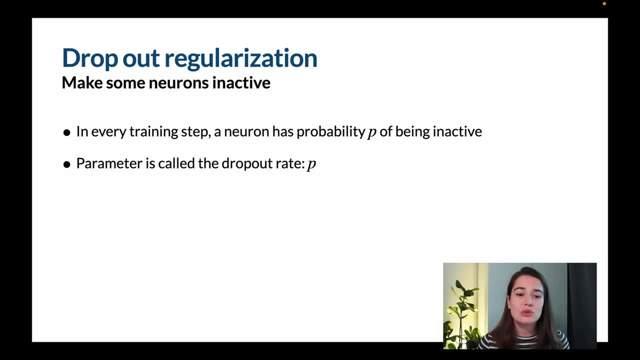 overfit the data because you're not really penalizing it enough. So this is one parameter that you need to tune while you're using regularization on your network. Then we have dropout regularization. What we do here is, in every training step, each neuron has a chance of P of being inactive, a probability P of being inactive. 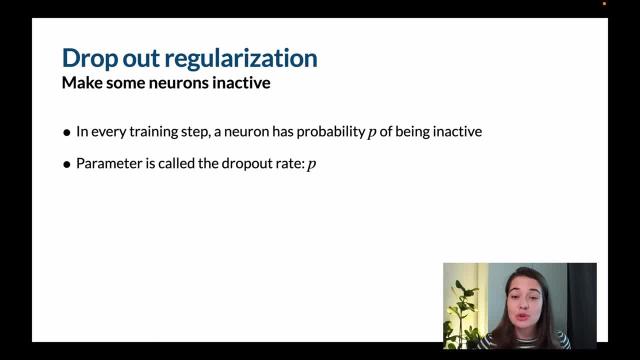 and that is called the dropout rate. It is something again we need to determine before we start training the network. Basically, what happens is: let's say, we have this network, we have two hidden networks, we have two hidden networks, we have two hidden networks. 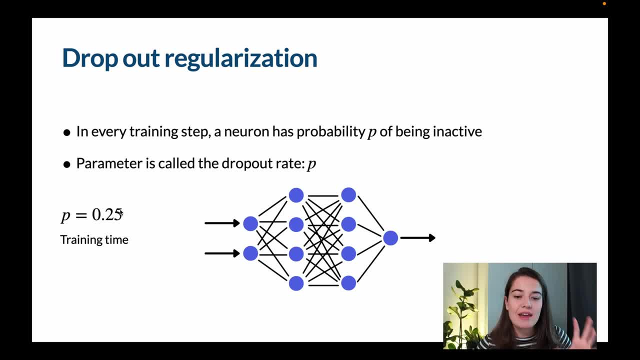 we have two hidden layers and we have four neurons each. If we say every neuron has a one fourth of chance of being inactive in a given step, then you might get you know one neuron missing from here, the first one and the second one. again some neurons missing from the first. 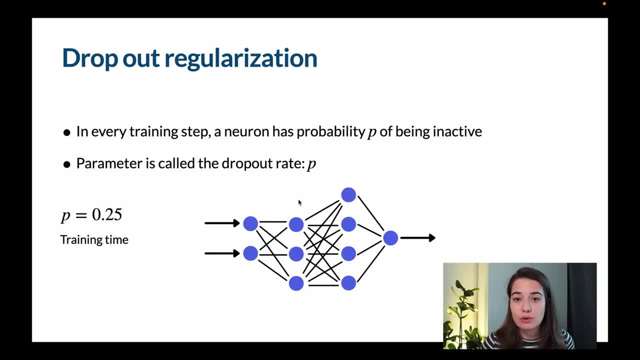 and the second. You might have more less than one fourth of all the neurons missing, or more than one fourth of all the neurons missing, of course, But on average, you're always going to have one fourth of neurons missing on your while you're using dropout regularization during training. 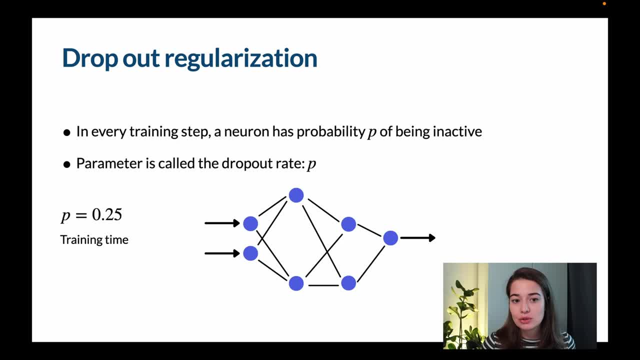 time And when you're using dropout regularization, you're going to have one fourth of neurons missing during training time. And one little trick here, one little thing that you need to understand about dropout regularization, is that when you're training some nodes or some neurons, 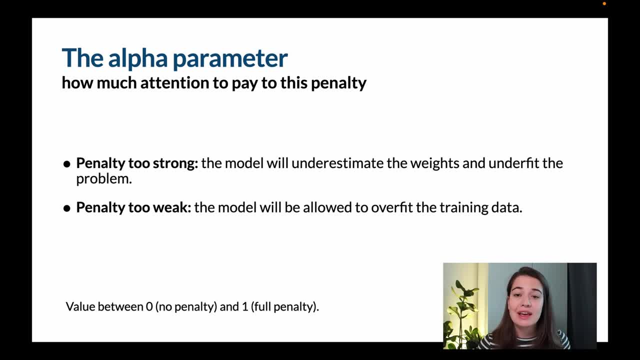 this penalty. so for l1 it was just the sum of all the weights, the absolute values of weights. for l2 it was the squared values of the weight, sum of squared values of the weight. so this alpha parameter tells us how much attention, attention to pay to this penalty. 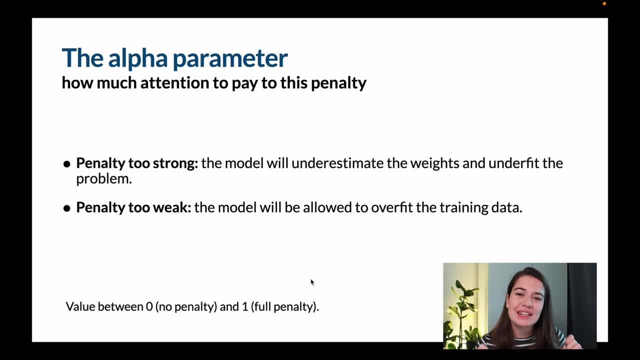 if you make the penalty too strong, then you're going to be regularizing a little bit too hard, and it is likely that your model might underfit your model. while you're trying to avoid overfit, you might get caught in underfitting. if you make the penalty too weak, though, then your model will. 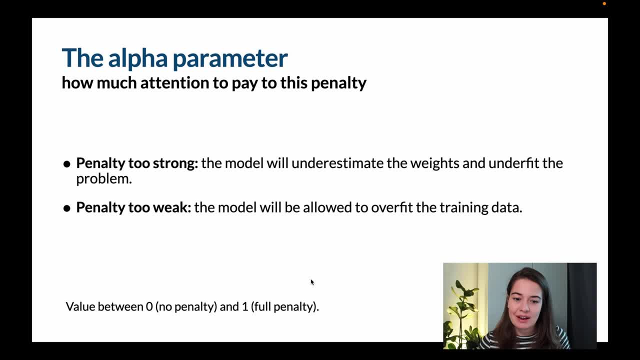 be allowed to overfit your model. if you make the penalty too weak, though, then your model will be allowed to overfit your model. if you make the penalty too weak, though, then your model will be fit the data, because you're not really penalizing it enough. so this is one parameter that you need. 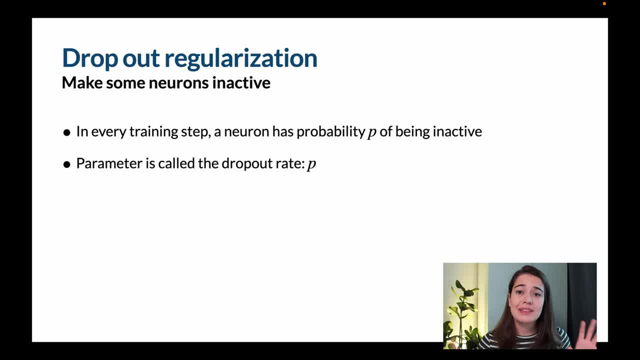 to tune while you're using regularization for on your network, then we have dropout regularization. what we do here is: in every training step each neuron has a chance of p of being inactive, a probability p of being inactive and that is called the dropout rate is something again we need to. 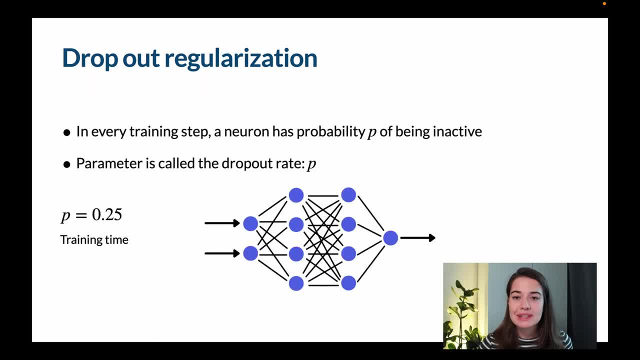 determine before we start trying training the network. basically, what happens is, let's say we have this network, we have two hidden layers and we have four neurons each. if we say every neuron has a one-fourth of chance of being inactive in a given step, then you might get, you know, one neuron. 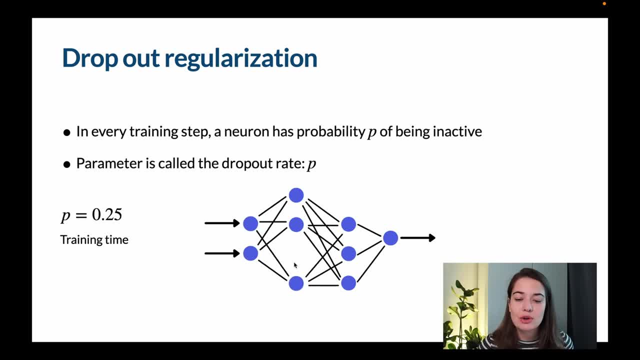 missing from here: the first one, the second one, again some neurons missing from the first and the second. you might have more. less than one-fourth of all the neurons missing, or more than one-fourth of all the neurons missing, of course, but on average you're always going to have one-fourth. 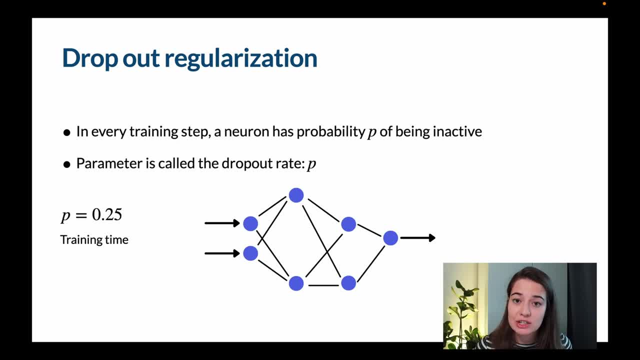 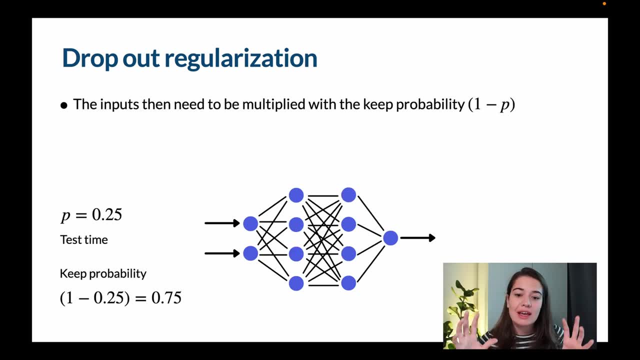 fourth of neurons missing on your while you're using dropout regularization during training time. and one little trick here, one little thing you need to understand about dropout regularization is that when you're training, some nodes or some neurons are going to be missing, but when you're testing, they're not going to be missing. so, as a result, what you need 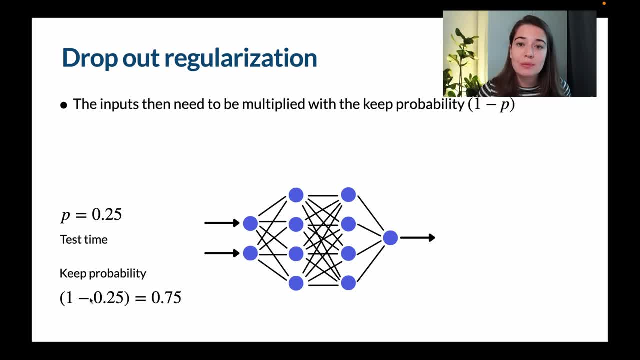 to do is to use something called the key probability, which is minus a dropout rate, and you need to multiply your inputs with this key probability because, if you think about it, because we are missing dropout rate, amigas amount of or, in this example, one-fourth of all the neurons on average during the training steps. 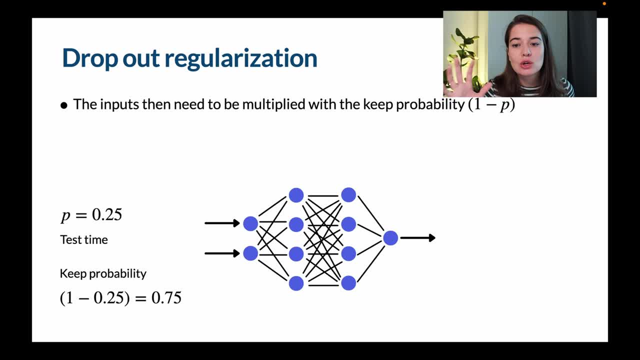 are going to be missing, but when you're testing, they're not going to be missing. So, as a result, what you need to do is to use something called the key probability, which is one minus a dropout rate, And you need to multiply your inputs with this key probability Because, if you think about 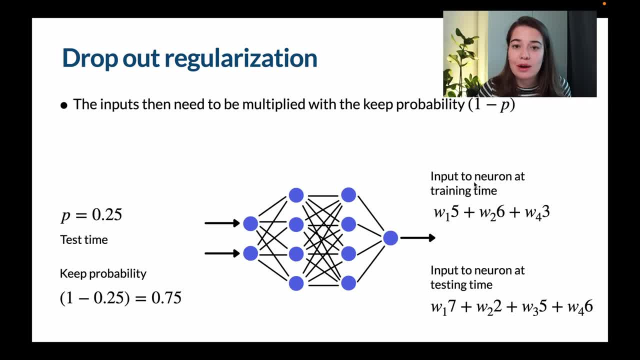 it because we are missing a dropout rate amount of, or we're missing a dropout rate amount of, in this example, one fourth of all the neurons on average during the training steps. we are basically going to be receiving three inputs, But for the test time. 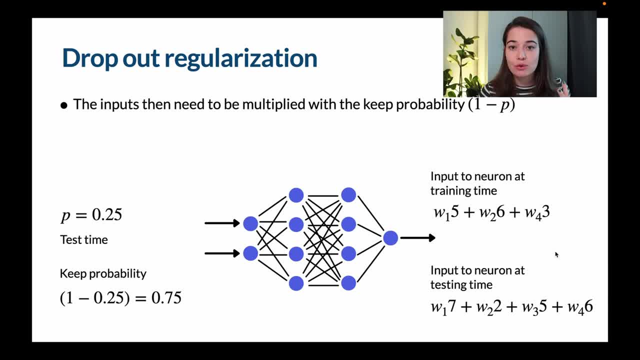 we are going to have all of our neurons and then we're going to be receiving four. So that's why we need to multiply our inputs with the key probability to make sure that the model is able to predict correct things and it's not really rigged in any way. And the next one we 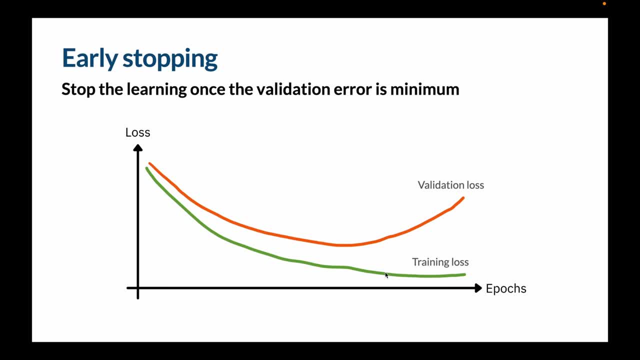 have is early stopping. We've seen this graph before: The more you train your network, the less ending loss is going to get. But after a while, validation loss is going to start getting higher And, as we said, that's the point- we start overfitting What you can do with early stopping. 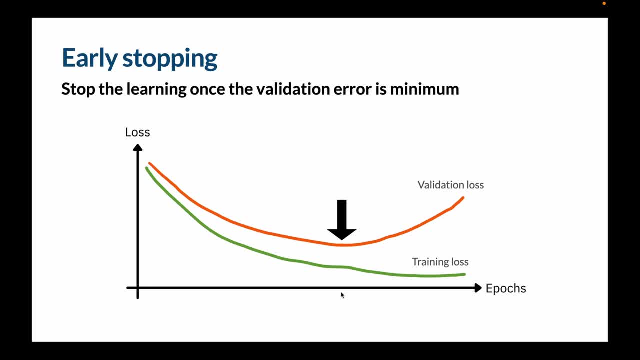 is to stop it at that point and say, okay, after 30 epochs my network starts overfitting. so I'm just going to stop the overfitting process, Though I have to say this is kind of a controversial technique. Not everyone agrees that this is a good way of dealing with overfitting. 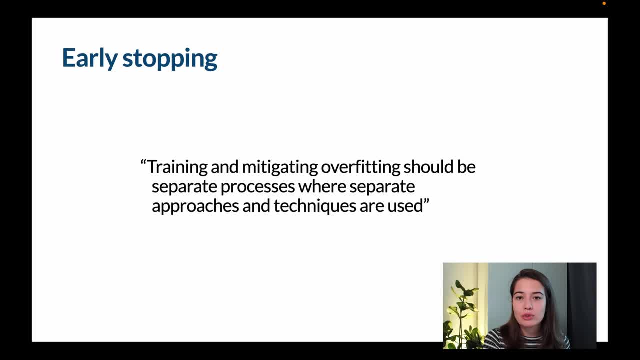 because what we want to do is we want to train our model, make sure that it converges to us the solution, and then have a separate process on top of it to deal with overfitting rather than stopping training early. Because combining these two processes 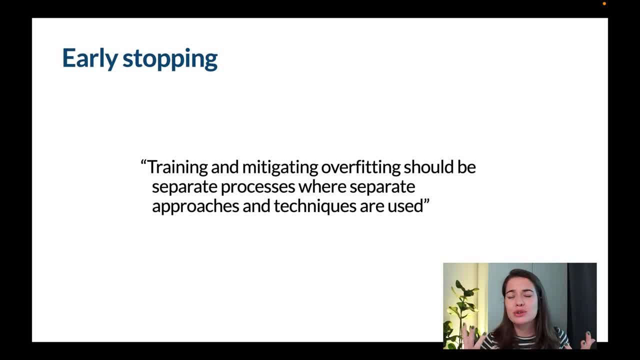 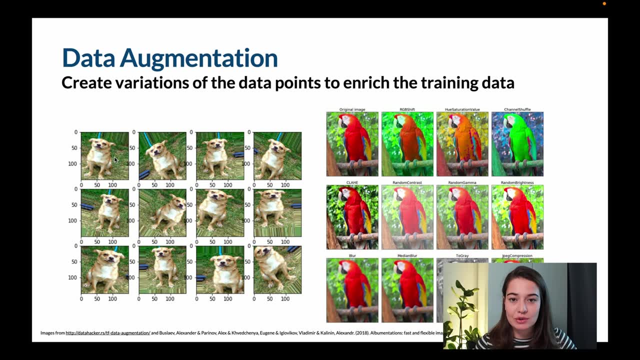 namely training and mitigating overfitting, will cause further confusion down the line, And the last technique that we have is data augmentation. So it's always a good idea to feed more data into your network, feed more different data into your network, but that might 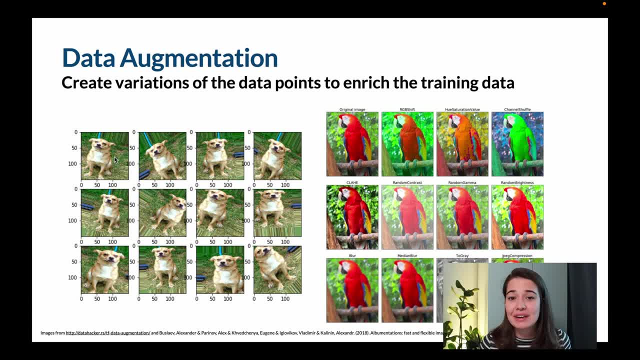 not always be possible for you- You might simply not have enough data, But especially if you're looking at images like these. let's say you are trying to understand or find dog faces in images, but you always have dogs sitting in a certain position, really straight 90 degrees to the. 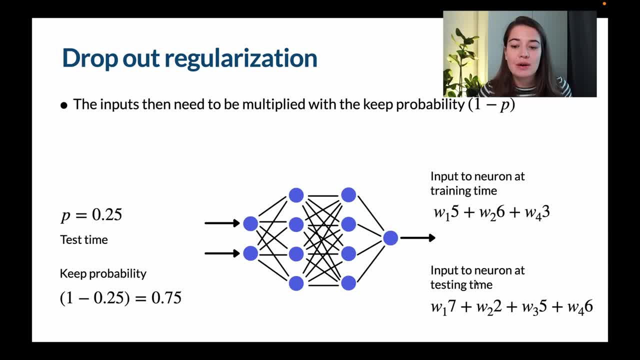 we are basically going to be receiving three inputs, but for the test time we are going to have all of our neurons and then we're going to be receiving four. so that's why we need to multiply our inputs with the key probability to make sure that the model is able to predict correct things. 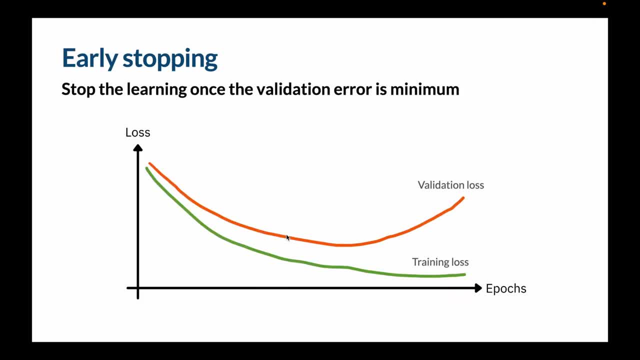 and it's not really rigged in any way. and the next one we have is early stopping. we've seen this graph before: the more you train your network, the less the training loss is going to get. but after a while, validation loss is going to start getting higher and, as we said, that's the point we start. 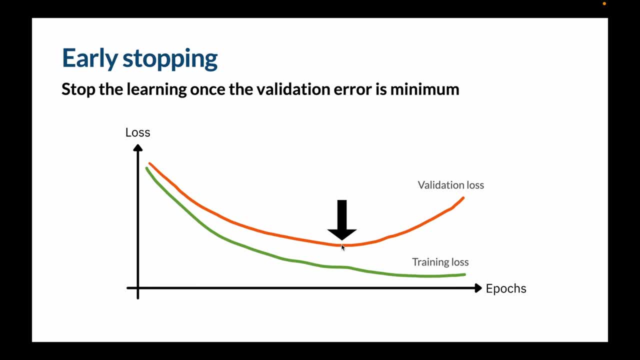 overfitting. what you can do with early stopping is to stop it at that point and say, okay, after 30 epochs my network starts overfitting. so i'm just going to stop the overfitting process, though i have to say this is kind of a controversial technique. not everyone agrees that this is a 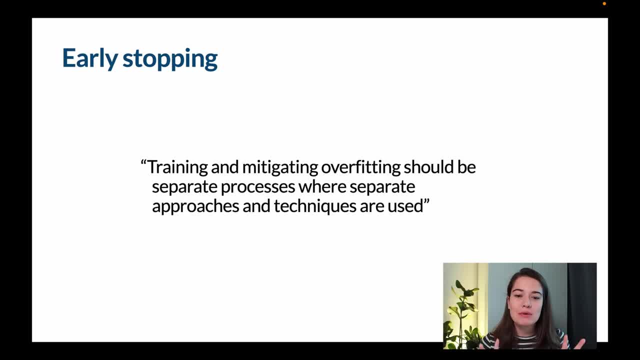 good way of dealing with overfitting, because what we want to do is we want to train our model, make sure that it converges to a solution and then have a separate process on top of it to deal with overfitting, rather than stopping training early, because combining these 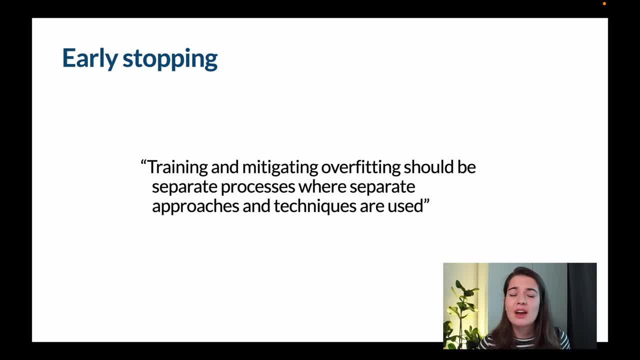 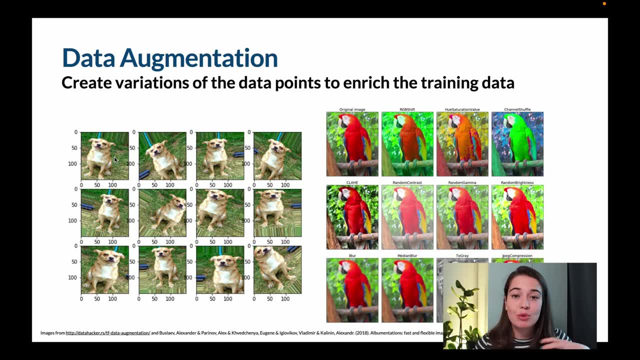 two processes, namely training and mitigating overfitting, will cause further confusion down the line, and the last technique that we have is data augmentation. so it's always a good idea to feed more data into your network, feed more different data into your network, but that might 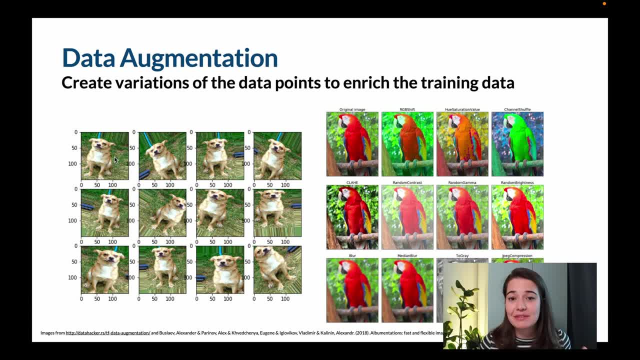 not always be possible for you. you might simply not have enough data, but especially if you're working with images like these. let's say you are trying to understand or find dog faces in images, but you always have dogs sitting in a certain position, really straight 90 degrees to the camera and looking directly into the camera. 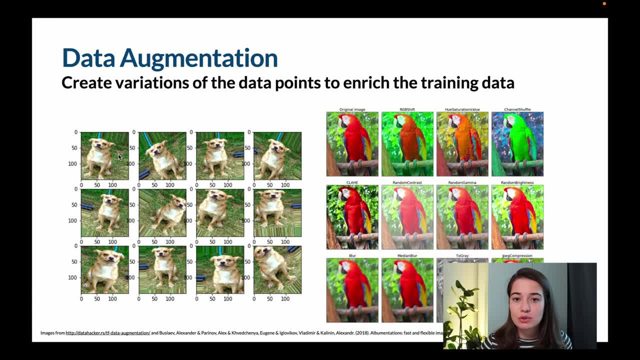 but you want your model to tolerate other pictures of dogs. you want it to be able to generalize to the real world. so what you can do is to flip or rotate or do other transformations to your images to basically have a more enriched training data or, if you want your model to be tolerable to the changes and exposure. 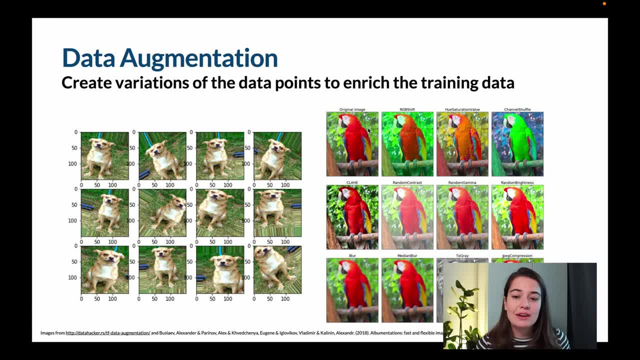 saturation or even just colors in general, then you can. you apply some other transformations to your data: increase the saturation, increase the hue, invert the colors, make it black and white, and then feed all of this data into your network so that it will be able to still recognize that.